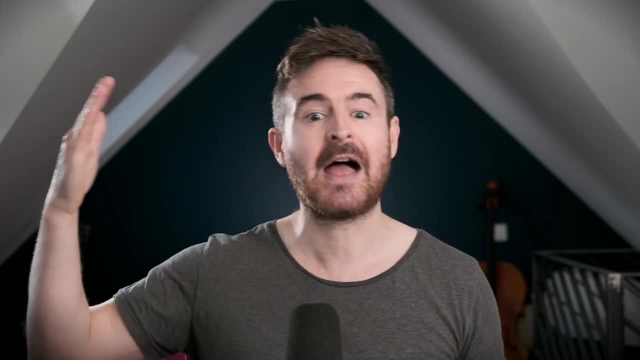 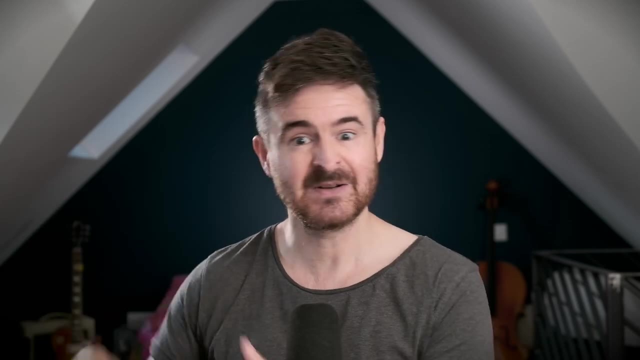 and Kath and we said: who's happy? Oh, maybe it's Anna and Beck who's happy, but not Kath. Then we just collect together Anna and Beck and we leave out Kath. That's a set. okay, The set. 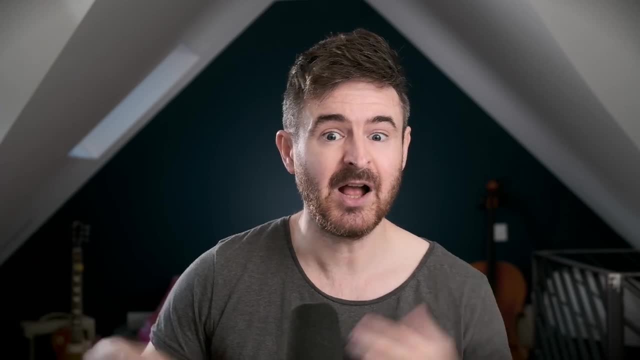 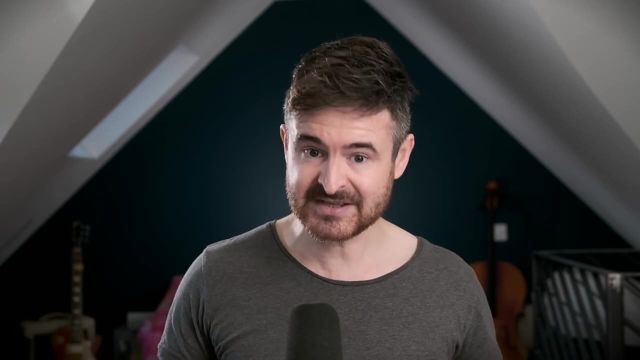 containing Anna and Beck, but not containing Kath. The domain too, that's a set right, It's a collection of entities. So the collection, the domain- Anna, Beck, Kath, that's another set. So we're already doing lots of stuff. 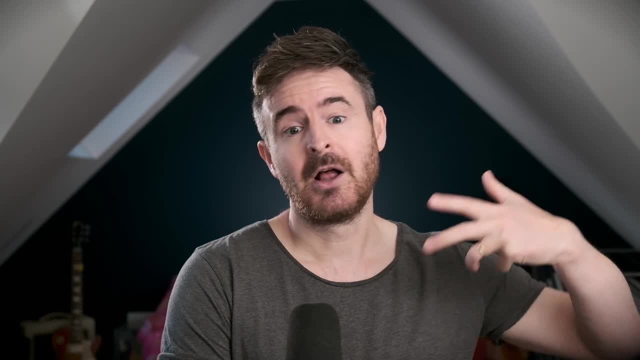 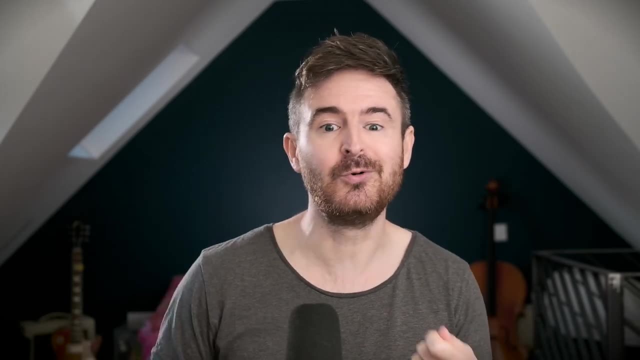 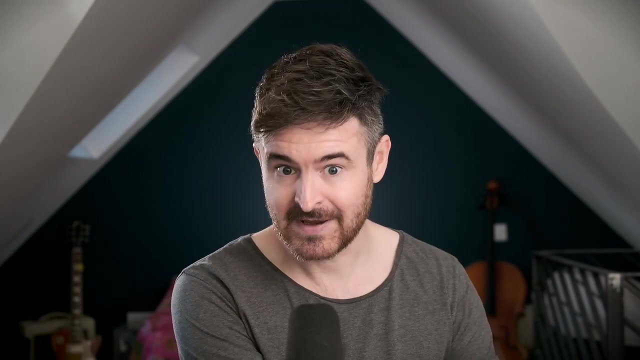 with sets, And set theory is basically the logical, mathematical theory setting out how collections work and how they don't work and giving us some tools for manipulating them, adding them together, that kind of stuff. So that's what we're going to be looking at in this video. 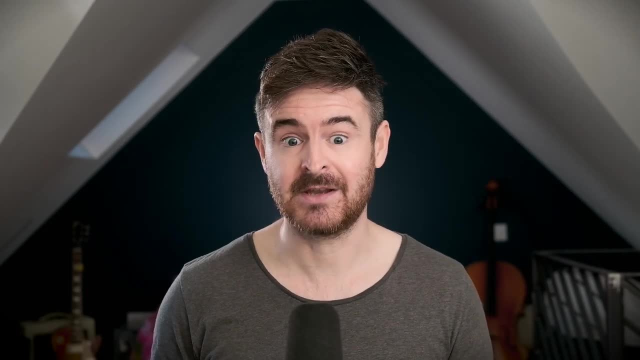 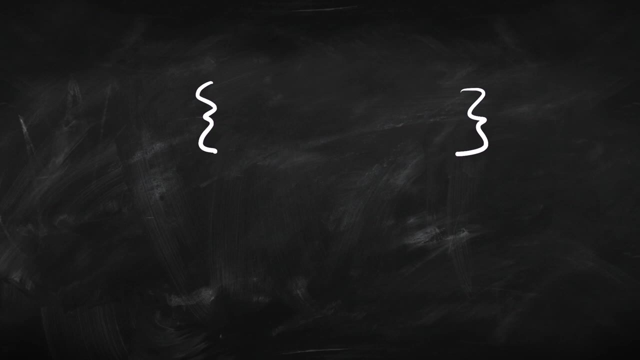 Okay, so let's start off with some basic ideas and basic notation. We're going to write sets down by writing curly brackets like this: curly braces- okay. We're always going to write sets like that And then sets have members. okay, So we might have three members: Anna and Beck and Kath. 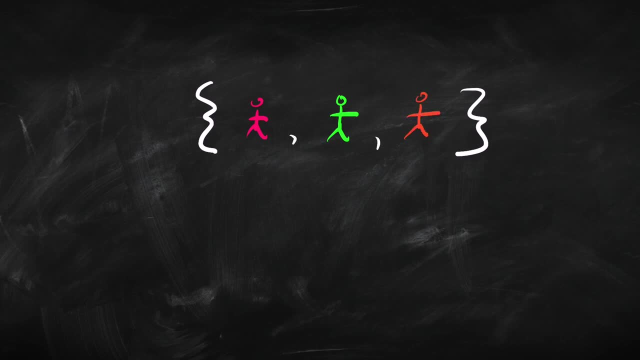 but we separate them out with commas. We've basically got a list of things in that set. Now it's a bit of a faff to always be drawing out the things in the set. So we're just going to use letters. We're just going to use A, B and C. The reason I've drawn out the pictures here is to 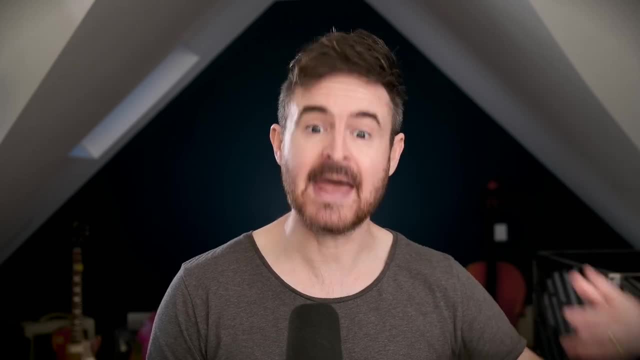 reinforce. it's the things in the set, So we're just going to use letters, We're just going to use A, B and C. It's not the names, okay. So the sets they're collections of things, not collections of bits of. 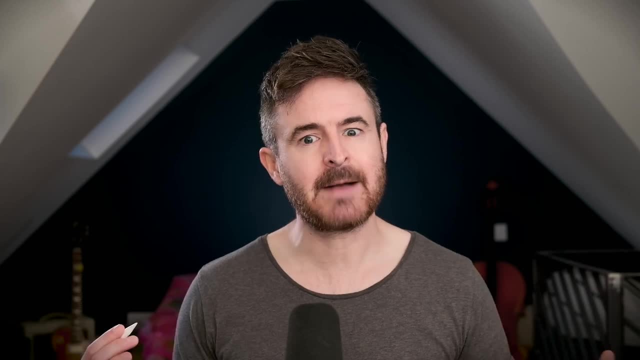 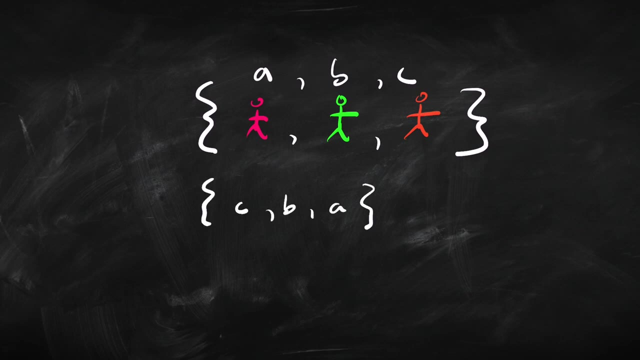 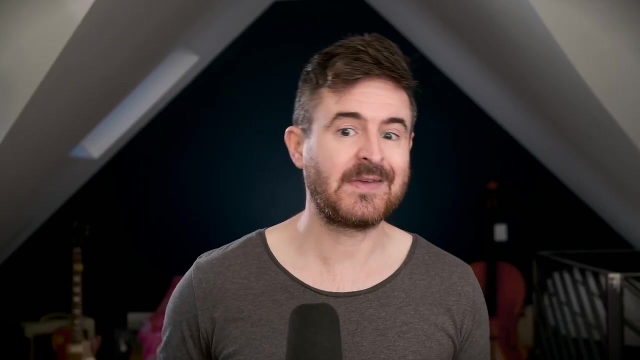 language. Now, a set is a collection in the sense that the order of things doesn't matter. So this set- A, B, C- is the same as this set. okay, I've written them down as two different ways, but it's the same set. They're identical. The only thing that's changed is the order in which. 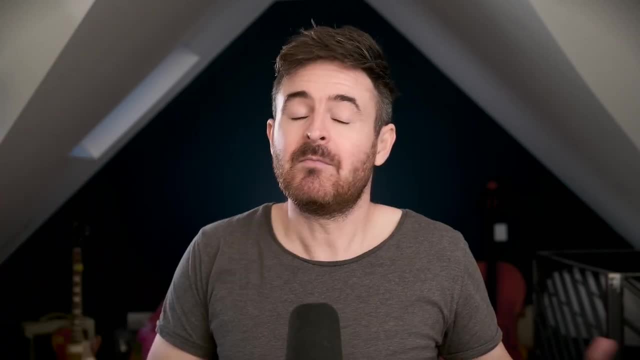 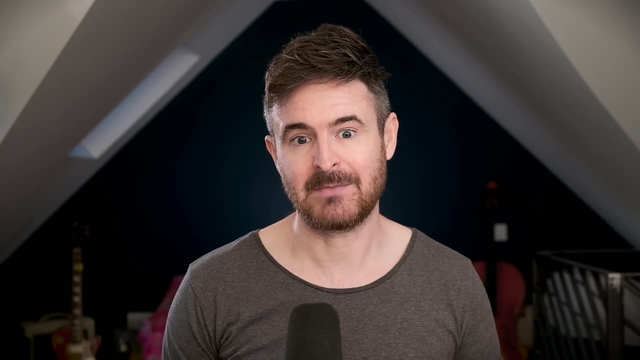 I've written them down, But because it's a collection, it's like a bag of things. the order in which I describe it It doesn't matter. Also, we don't have repetitions in the set, okay, So if I collect together, Anna. 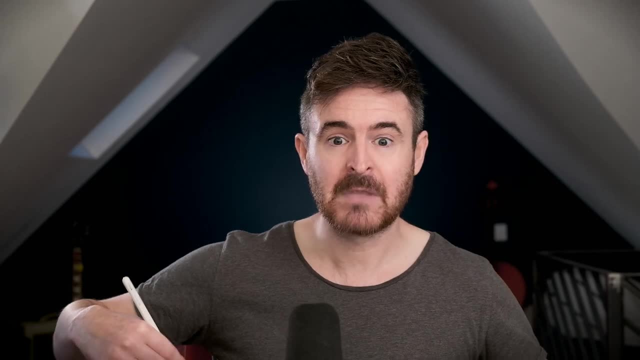 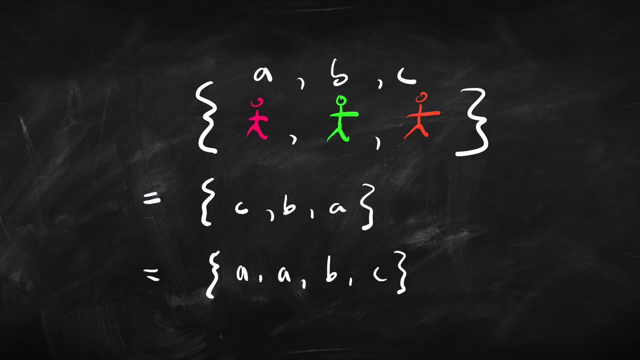 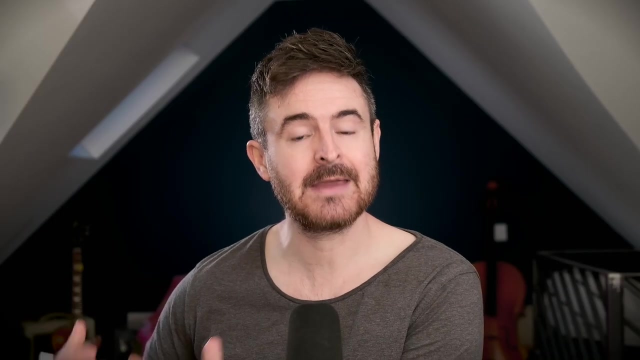 and Beck and Cath and then Anna again. it's the same as just collecting Anna and Beck and Cath. So this is also the same set as this one. In this third example I've written down Anna twice, so I've kind of described that bit of the set twice, but it's the same set. So basically, 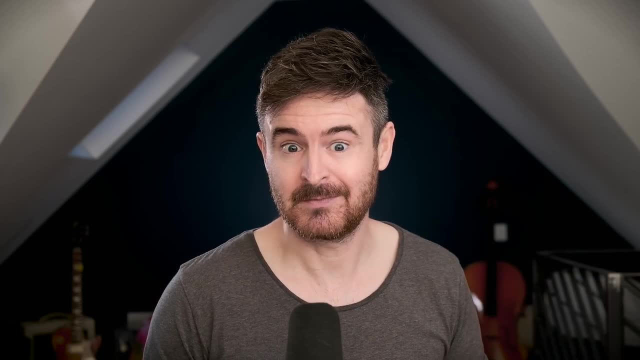 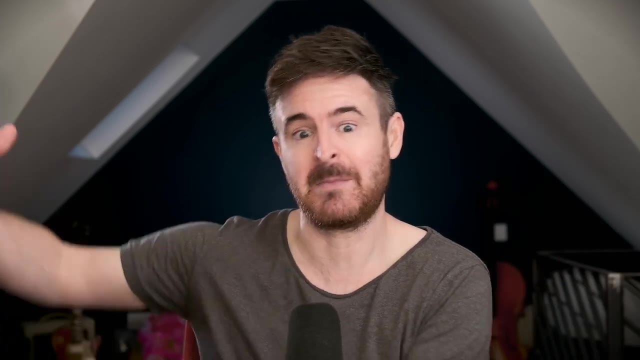 we ignore repetitions and we ignore the order. So in that sense it's different from a shopping list, because if I do my shopping list the order might matter, Repetitions might matter. It might mean I want two of those things. 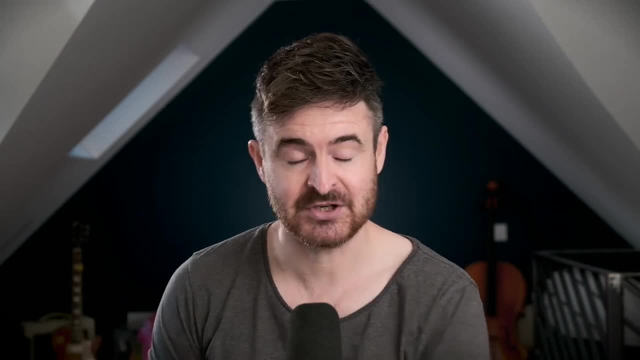 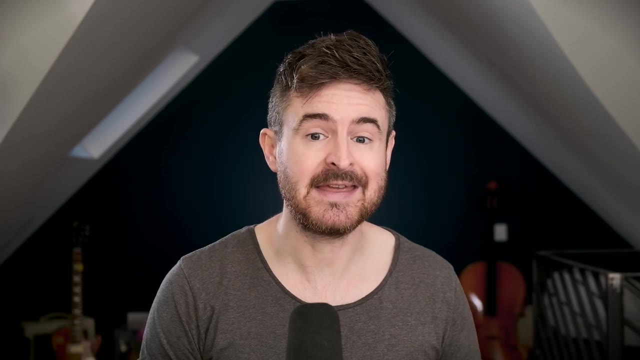 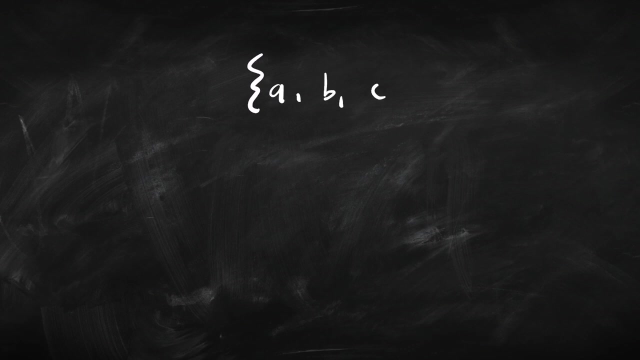 It's not like that for sets. Order doesn't matter, Repetition doesn't matter. We ignore those things. Probably the most important concept when we're dealing with sets is the idea of membership. They're members. So in this set- A, B, C- we've got three members. Some people call them. 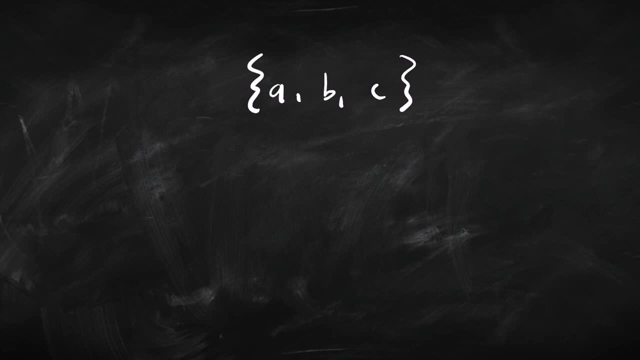 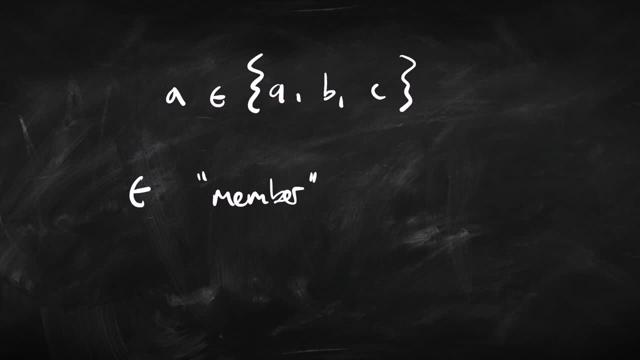 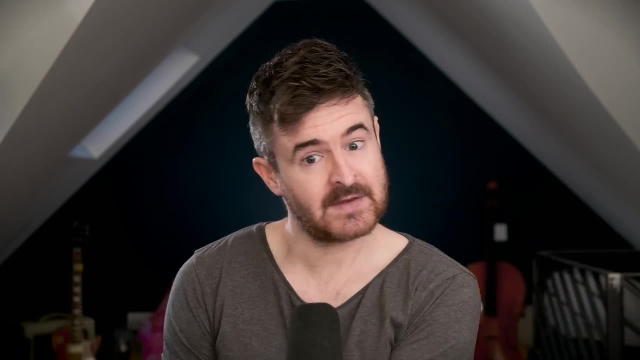 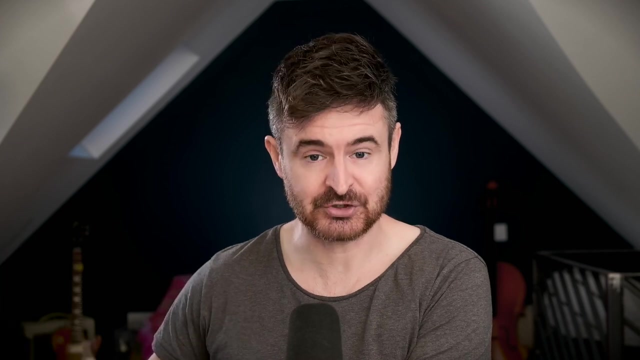 You can also write down: B is a member of that set. C is a member of that set. Okay, That's going to be one of the most important concepts. when we're dealing with sets- All of the other things that we look at- we can basically define all of the other concepts using membership, plus some logic. 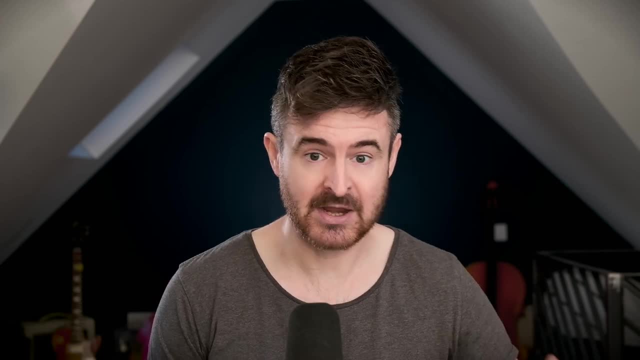 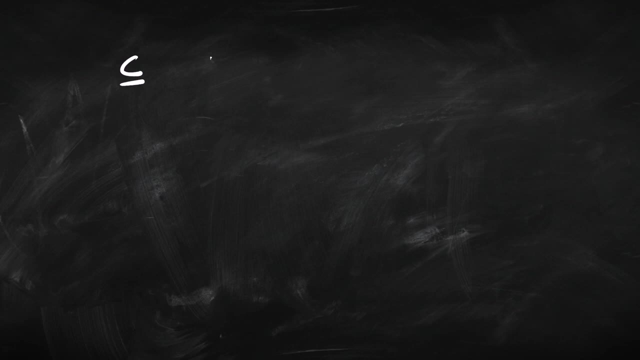 Okay, Let's have a look at some of the other concepts that we're going to be interested in And we're going to try and talk through how we could define them using membership. Okay, So here we've got a relationship between two sets, a relationship of inclusion. 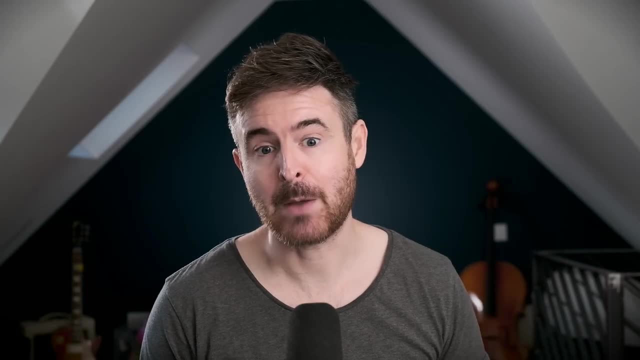 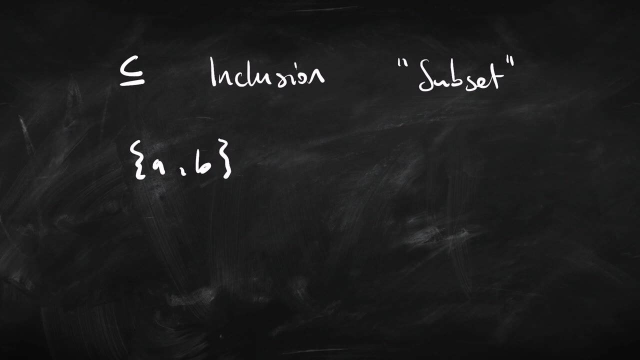 One set includes another, Or a different way of saying it would be that one set is a subset of another. So let me give you an example. Here's a set Just got A and B in it. That is a subset of the set. 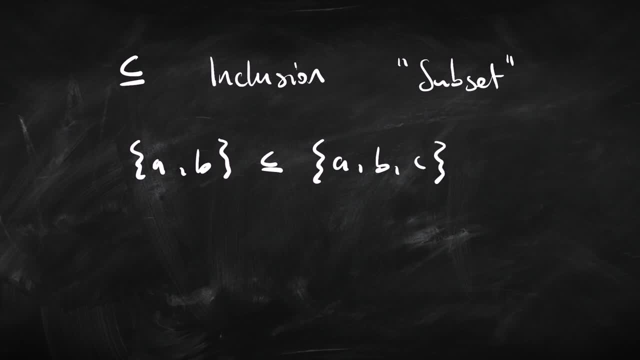 that we saw before: A, B, C. Okay. Now, what that means is that everything in here also appears over here. Okay, So this set on the right includes the one on the left. This one is a subset of this one, So if we were to define this just using 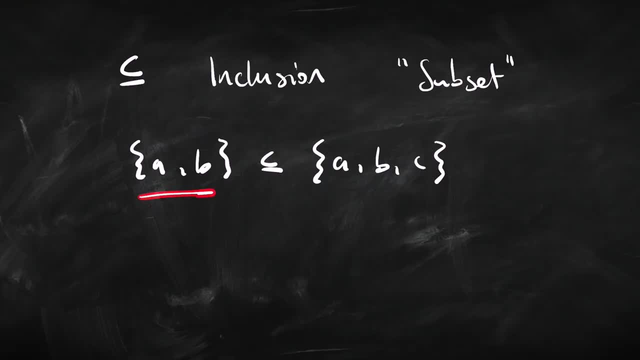 membership and a bit of logic. what you would say is: everything that's a member of this is also a member of this. So, for all X, if X is a member of this, then X is a member of this. Okay, That's. 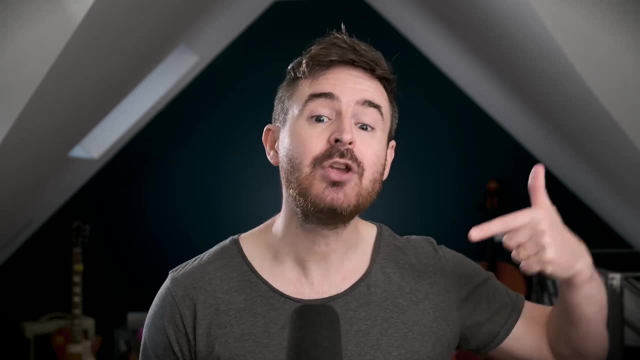 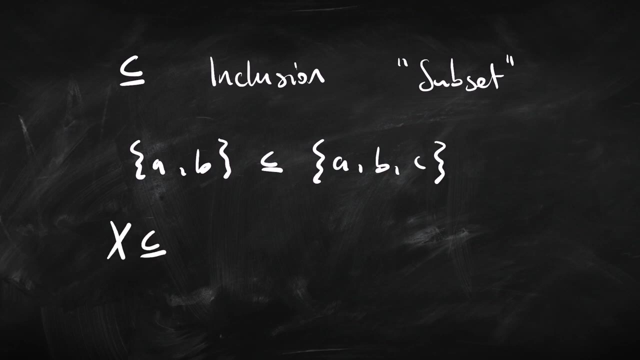 a logical definition of the subset relation in terms of the membership relation. So let's write that down. Suppose we're talking about two sets, X being a subset of Y. So let's give a definition of that. Let's say, for all things, 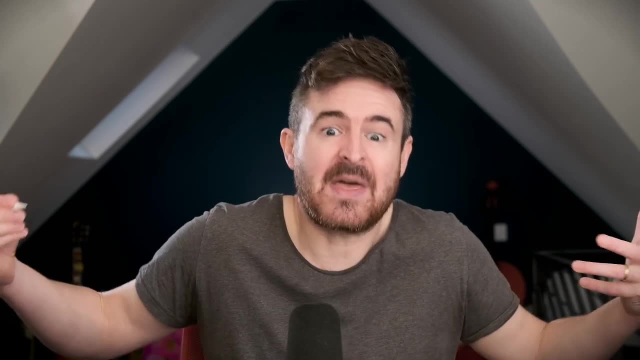 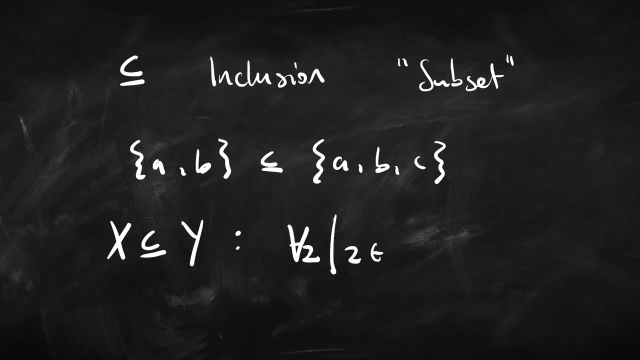 Z- and I'm using Z here because I've already used X and Y, even though they're capital X and Ys and a little Z. it kind of gets a bit confusing to say it out loud. So, for all things Z, if Z is a member. 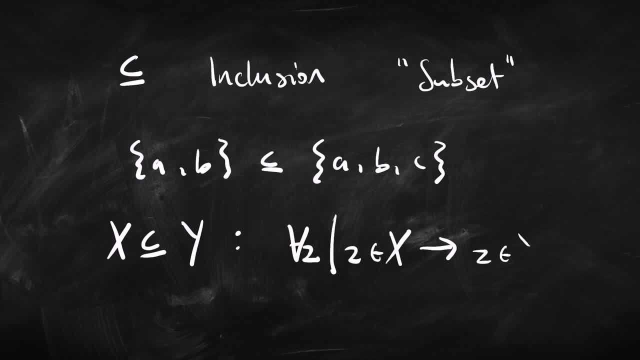 of X, then Z is also a member of Y. If our thing is in here, then it's also in here. So A is in here, It's also there. B is there, It's also there. C is there, but not there. But that doesn't matter. 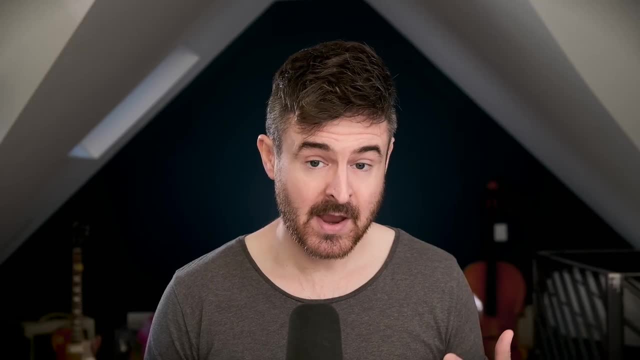 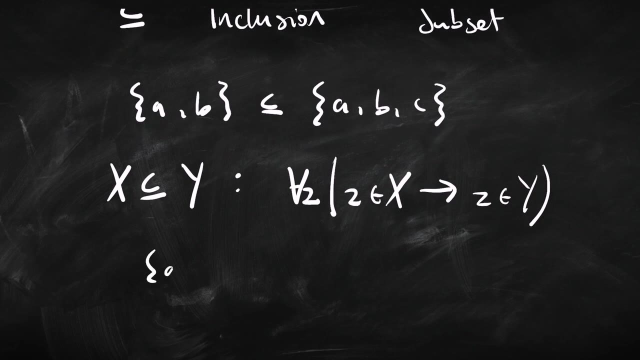 because we don't require the things here to be here. Here's something to bear in mind with this definition. It says that everything in the first set is also in the second. So what about this case? Is that a good case of inclusion? Is that a good case of a subset? Well, everything here is over here, Yep. 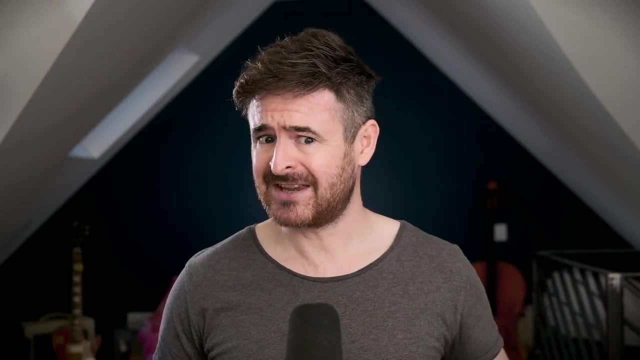 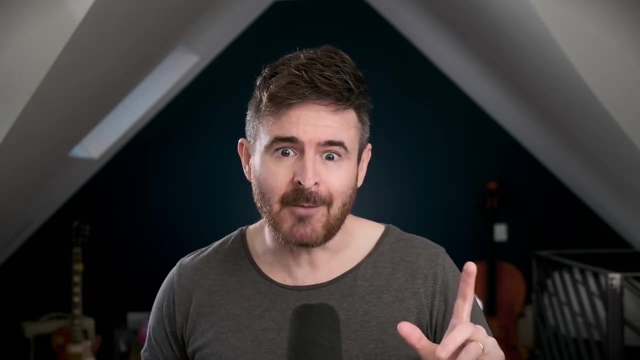 that's true because they're the same set. But that might seem a little bit weird, right? Because when we're talking about a subset or inclusion, we normally think of the one as being bigger than the other. But when we're talking about a subset or an inclusion in set theory, in logic, we always 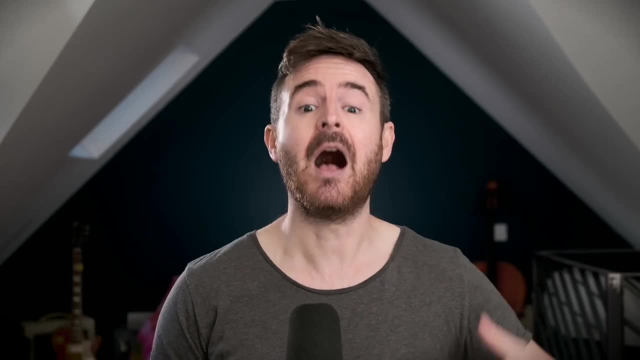 think of the one as being bigger than the other. So we're talking about a subset or an inclusion in set theory. But when we're talking about a subset or an inclusion in set theory, we normally think of the one as being bigger than the other. So we're talking about a subset or an inclusion in. 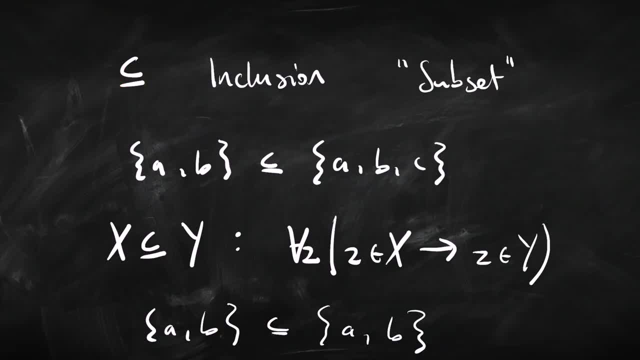 set theory, And that's why we have this little line under the symbol here. It's kind of meant to indicate the, And also it includes the identity case, because this is kind of like a little equal sign down the bottom here. So this is our basic notion of subset. We can also have 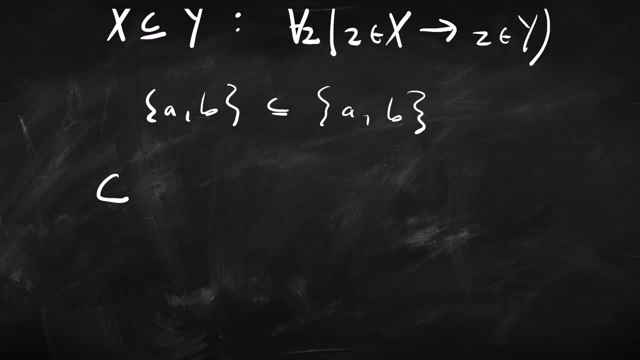 the notion of what we call a proper subset. So that's where we write it like this: So we have a subset or a subset, We can also have a subset or a subset. So we have a subset or a subset. We can also have a subset or a subset. So we have a subset or a subset, We can also have a subset or a subset. 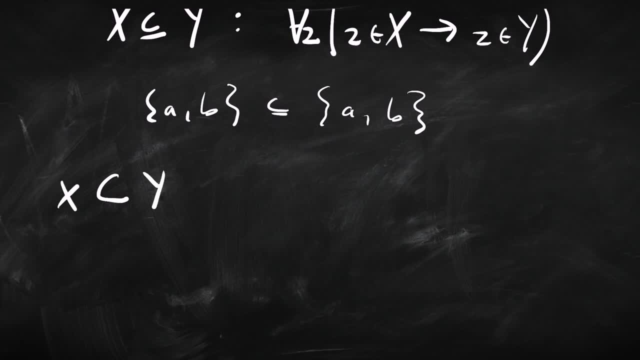 And there we're saying: everything in X is also in Y, but they're not identical. Okay, so there's going to be something over in Y that we don't find in X. So that is like the case where we've got A and B over here and that's a proper subset of A, B, C, But we think of that as a derivative. 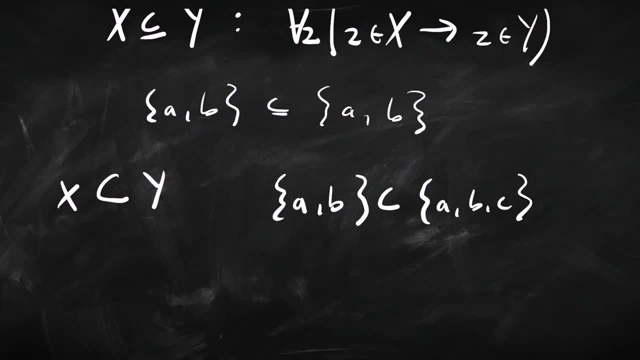 concept, because the easiest way to define this is by saying: well, it's a subset In the kind of previous sense, but they're not identical. Okay, so it's kind of like a compound concept. They're a subset, but they're not the same thing, So there's got to be something here. 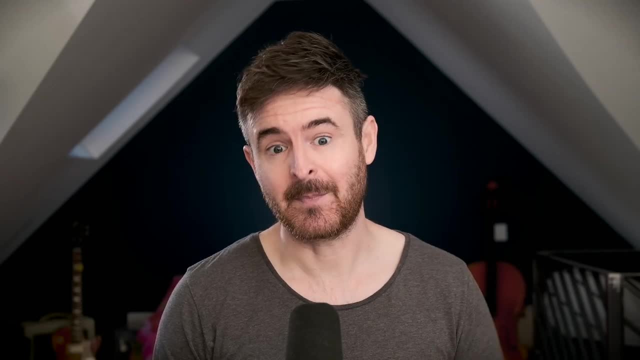 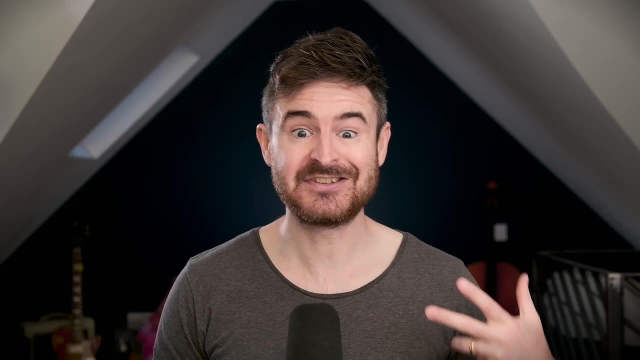 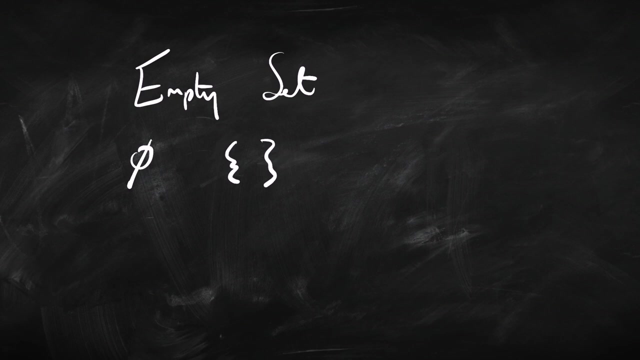 that isn't here. One more super important concept that we're going to see right the way through this stuff on set is the idea of the empty set. This is the set that doesn't have any members. We can write it down like this: Okay, so this is the two set brackets, but with nothing in the middle. 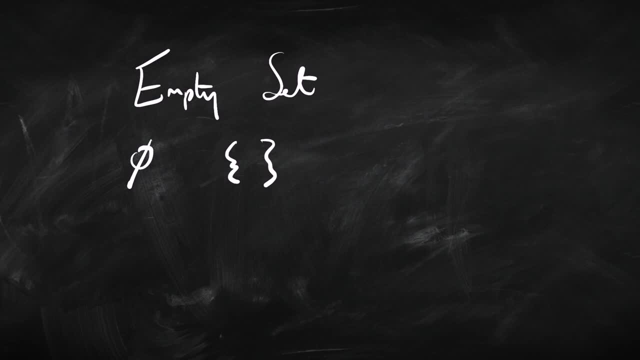 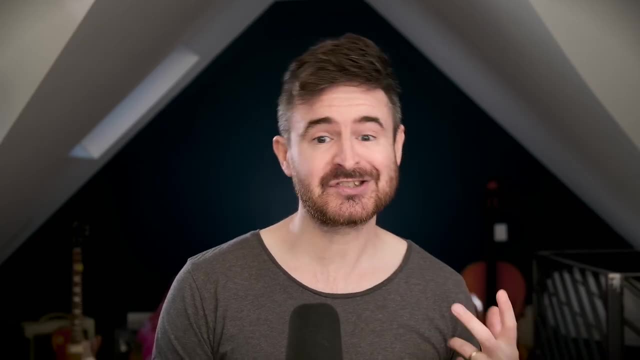 This one's quite good because it kind of shows that it's the empty set, because we're writing a set and we're not putting anything in it. but you'll often see that symbol as well. Okay, so philosophically the empty set is kind of like a puzzle. It's kind of like the number zero. So if numbers are meant, 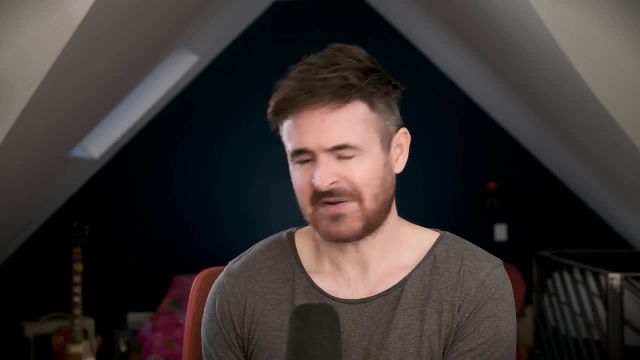 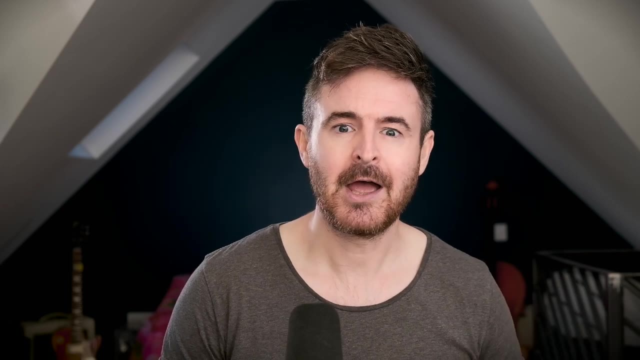 to represent quantities of things, then you might think: well, if I've got nothing of something, then I haven't got anything, so they shouldn't be a zero quantity. But what we know from doing maths is that it's kind of really useful. So if I've got nothing of something, then I haven't got. 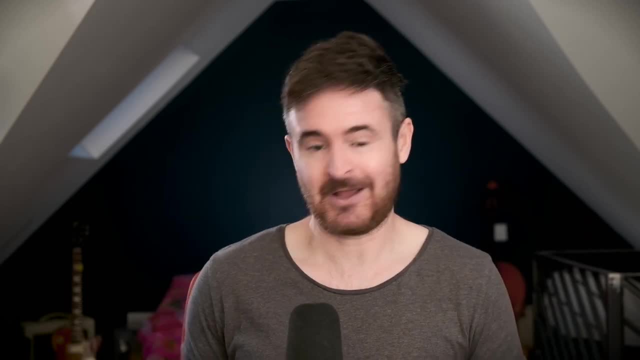 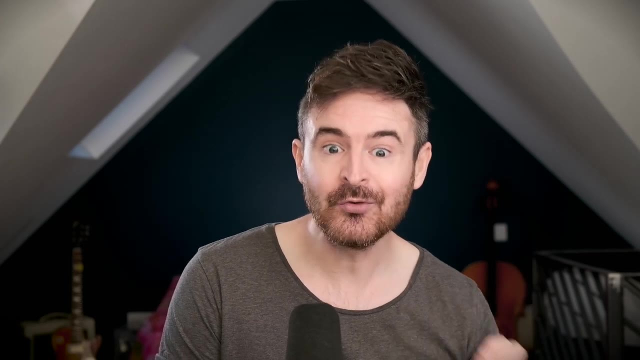 anything. But what we know from doing maths is that it's kind of really useful to have zero as a number. Otherwise we're kind of doing like subtraction and we kind of get confused if we're doing like one minus one. So we need this number. Zero is a really useful concept to have. 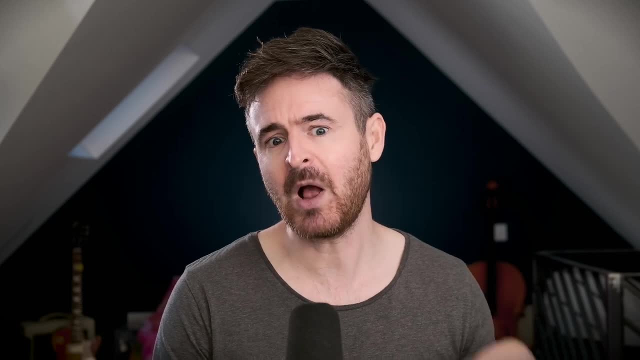 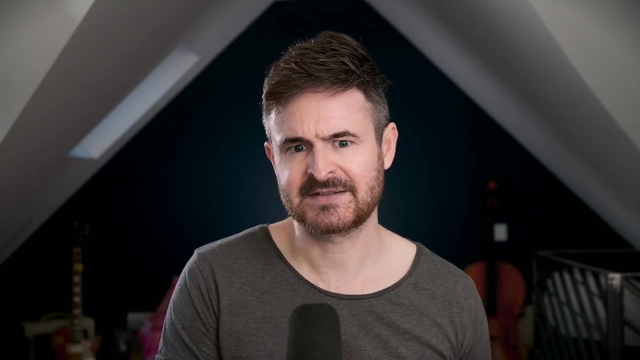 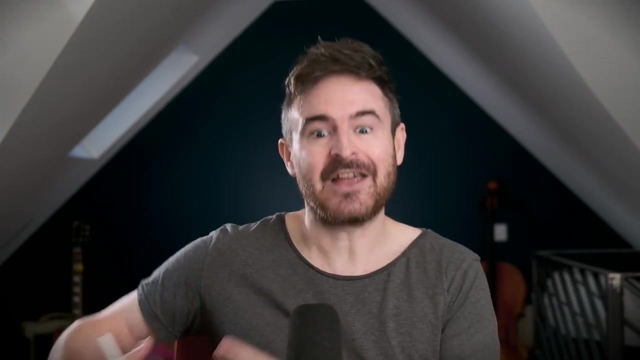 even if it doesn't correspond to a quantity in the real world. Exactly the same goes with sets, right? So we start off thinking that a set is a collection of things. So you go: oh, it's a bit weird to think of an empty set, a collection of nothing, But it's kind of like once we get this: 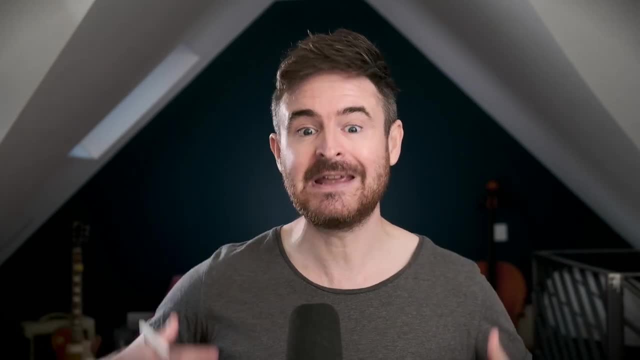 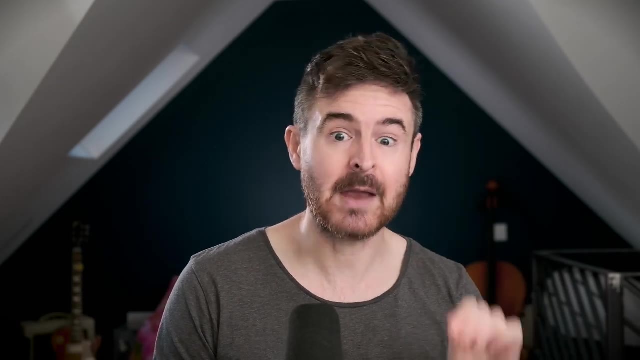 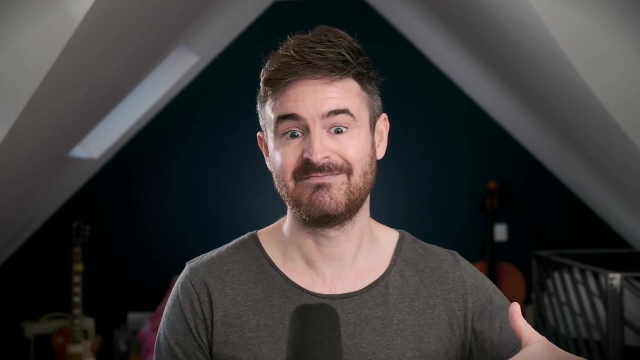 calculus of sets going. once we get the theory going, it's really useful to have a kind of a zero, something that corresponds to the number zero. So we definitely want to have the empty set in there. Okay, The empty set is defined as the set that has no members, So nothing is a. 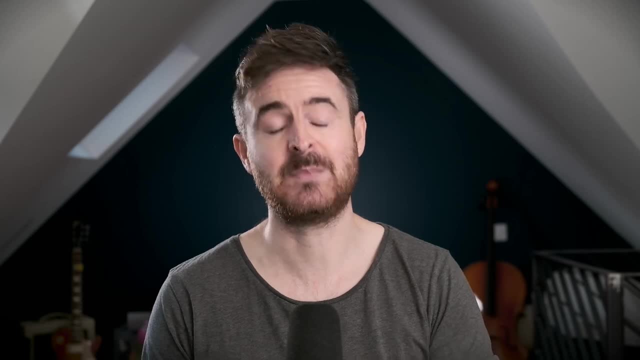 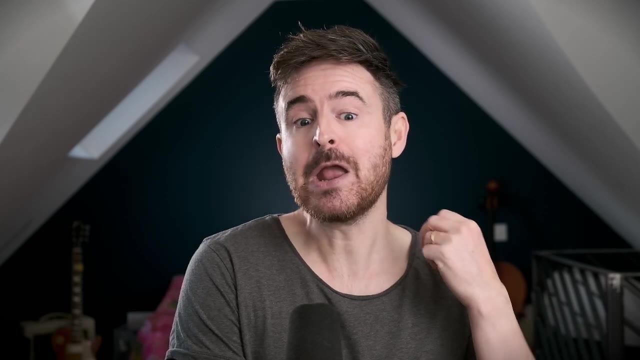 member of it For everything. it's not a member of the empty set. That's a logical definition of the empty set in terms of membership. Pretty easy to see that from this there is only one empty set, right, Because if imagine there was two, well they would both have no members. 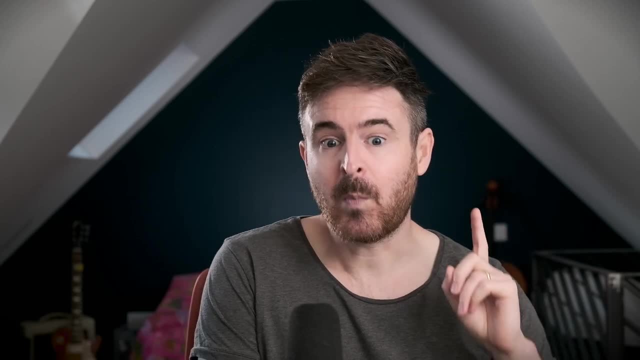 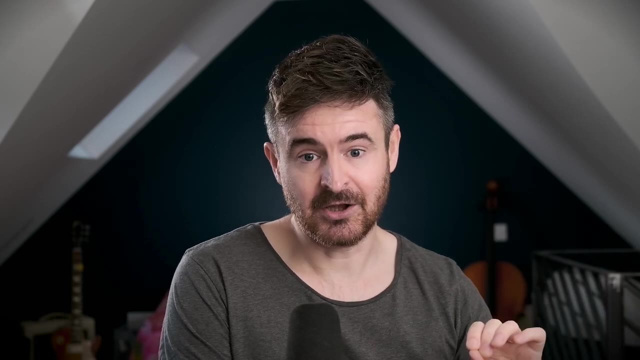 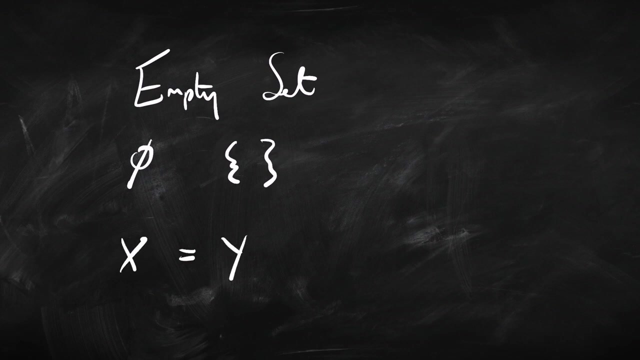 So they would be the same. Because here is a really important thing about sets in general: not just the empty set, but all sets: Set A and set B are identical when they have the same members. So I'm just going to say that again: If we've got sets X and set Y, they're identical if, and only if, 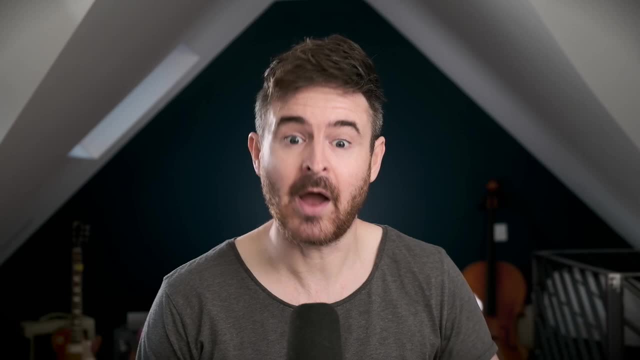 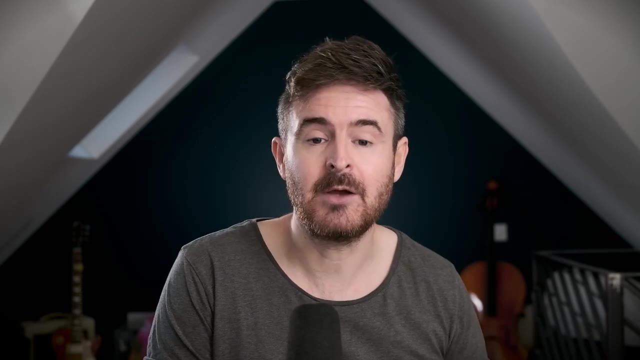 all of the things in X are in Y and all of the things in Y are in X. They have the same members. Okay, So a logical definition of identity between sets can be given in terms of membership For all things Z Z's in X, if, and only if, Z's in Y. 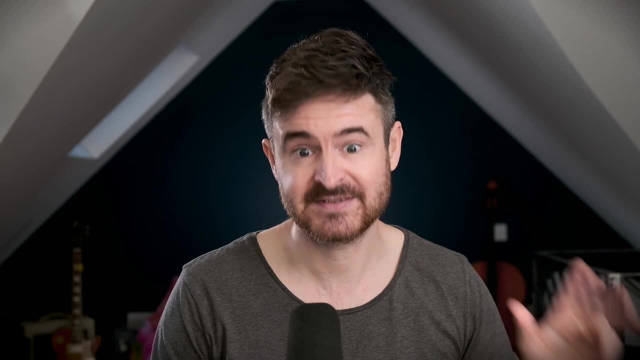 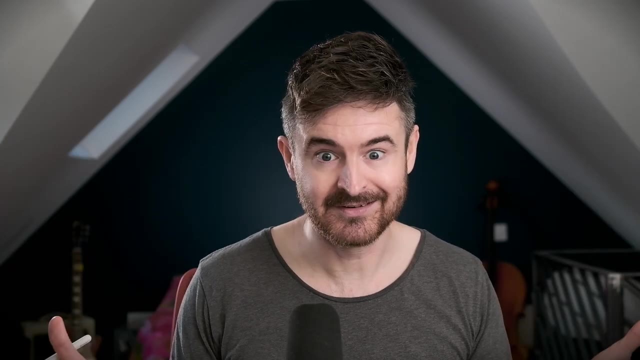 If that's the case, then X- Y are the same set. So, going back to the empty set, suppose we had two empty sets. Well, they would have the same members, right? Ie, none, So they would be the same set. That's why you can't have two empty sets. So we can talk about the empty set. 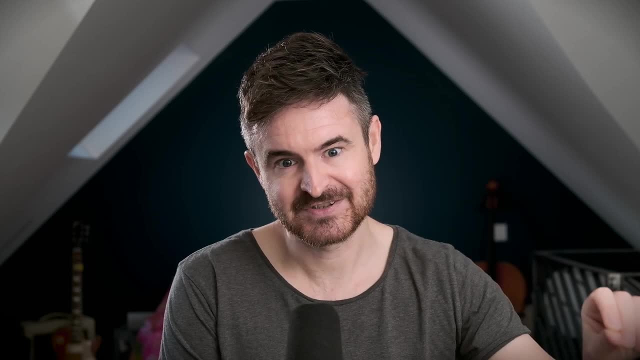 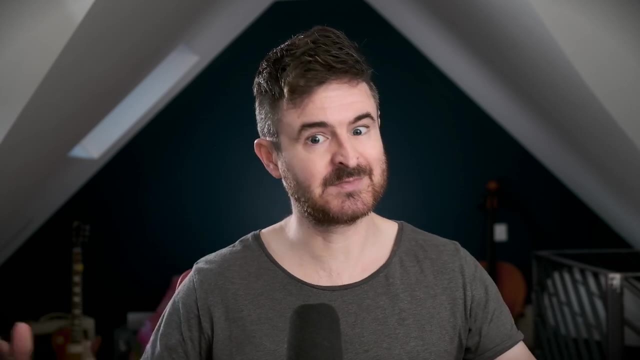 the one and only The unique set with no members in it. Let's talk some operations on sets. These are ways of forming new sets from old sets. So I'll give you some sets and we can do stuff to them to form new sets. 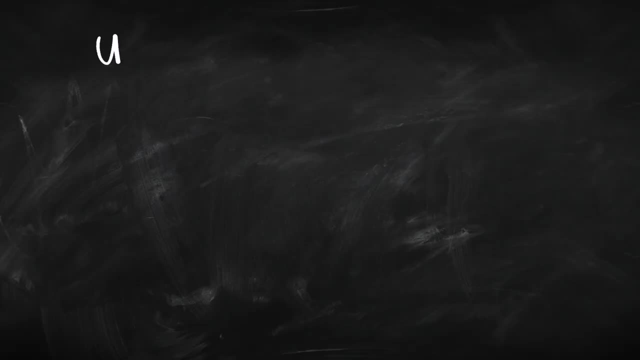 There's going to be four operations that we're interested in. There's the union of two sets, which we write like that, So X union Y. There's the intersection, and we write it like that. There's the complement- Different ways of writing that. 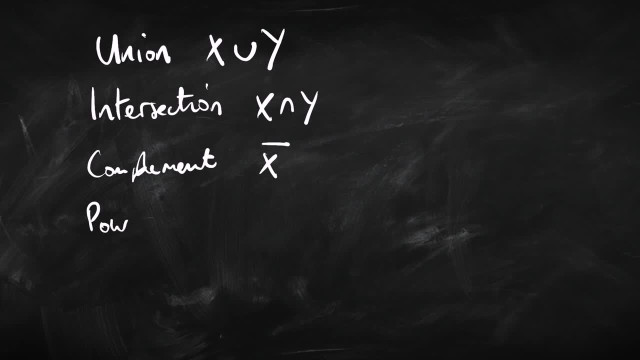 but that's the way we're going to do it, Putting like a bar on the top of it And there's the power set, And we're just going to write that with a P. How do you remember all these symbols? Well, union looks like a U, Intersection. Well, 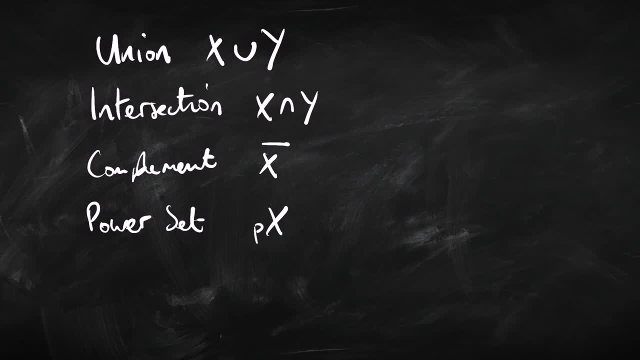 that's the one that looks like union, but it's not union, So it's intersection Complement. This is kind of like negation, So it's a bit like the negation symbol, And power set is a P, So you 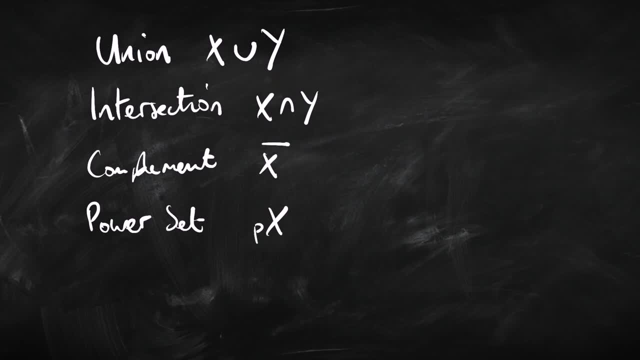 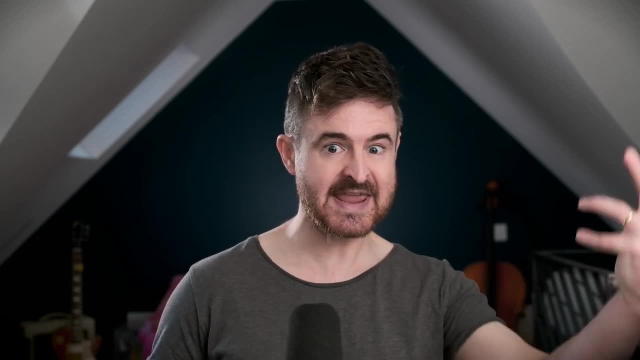 can remember that one. What do they all mean? The union of the two sets is the set that contains everything in X plus Y, Everything in Y but nothing else. So we take X, we take Y and we squidge them together. 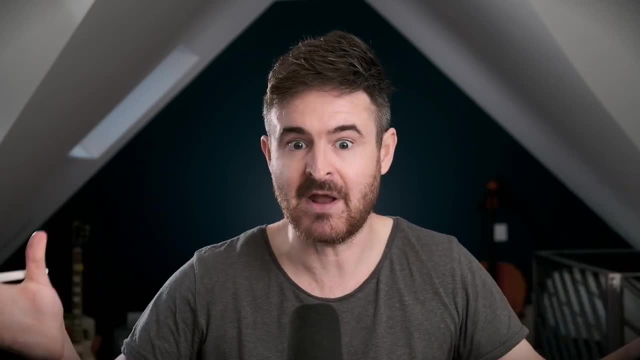 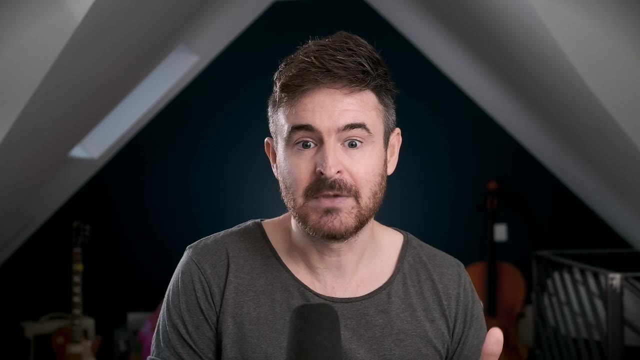 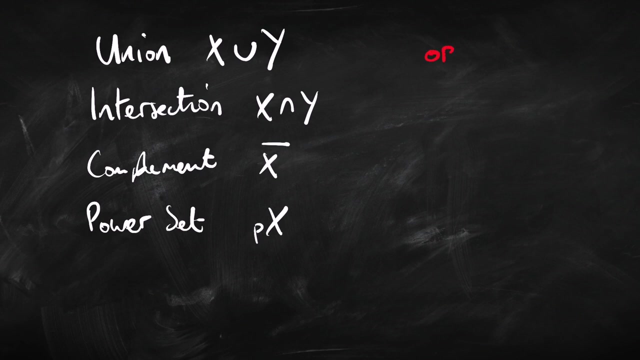 So the new set is everything in X and everything in Y, but nothing else. So a logical definition of the union of X and Y would say: something is in that union, just in case it's in X or it's in Y. So union is a little bit like or Something is in here if it's in X or it's in Y. 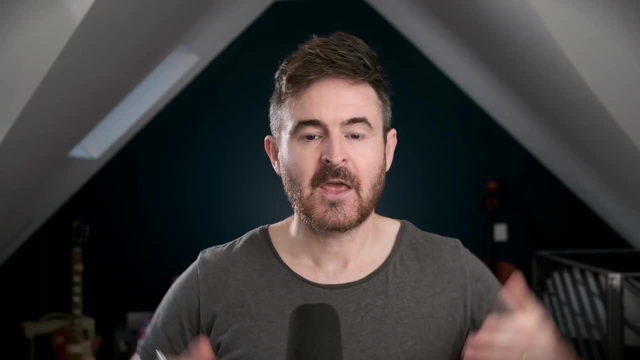 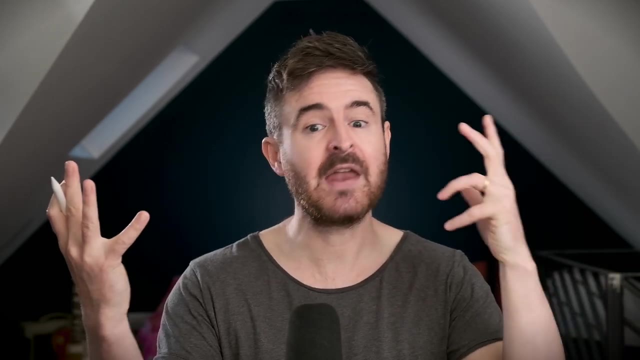 Intersection. So union is a little bit like, or Something is in here if it's in X or it's in Y. Intersection, on the other hand, is like: and The intersection of X and Y, on the other hand, is all of the things that are in both of them. So I look at X, I look at Y and if there's anything, 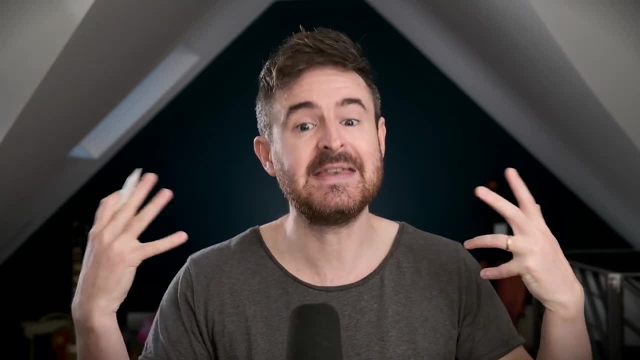 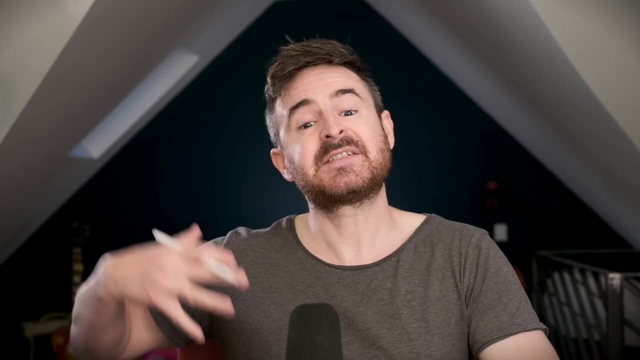 common to both sets, then that thing is in the intersection of them. The complement of a set is all the things that aren't in that set. So if you think about it, that has to be relevant to some kind of background universe of things. So we have to fix all the things we're talking about. 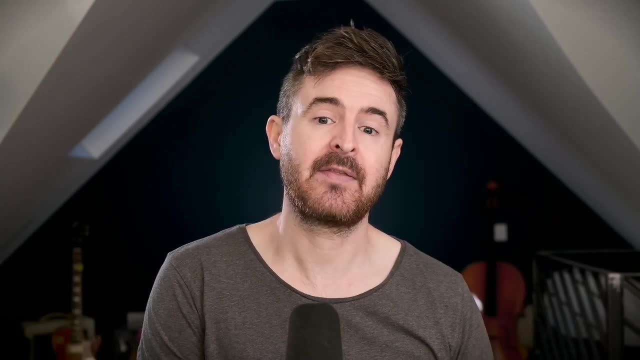 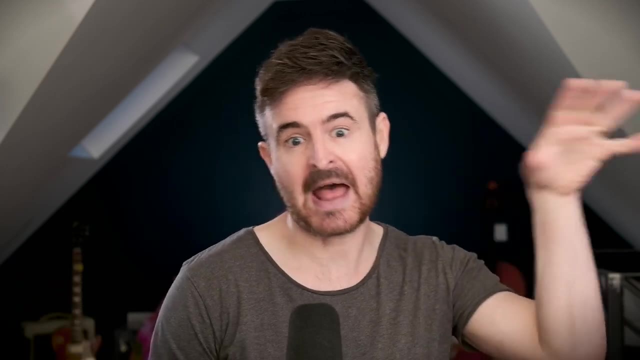 So let's say we take our domain to be Anna, Beck and Kath. Relative to that, if I give you a set then you can calculate the complement. So let's have the happy people. So that was Anna and Beck, The complement of the. 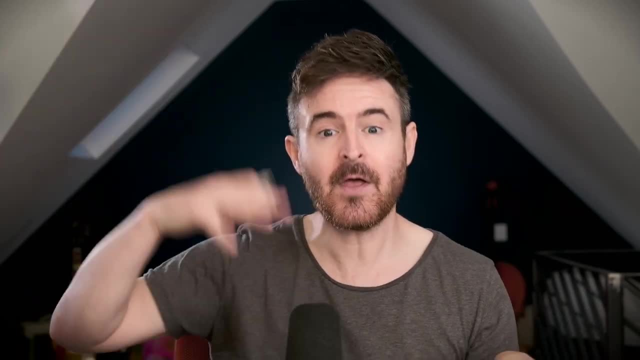 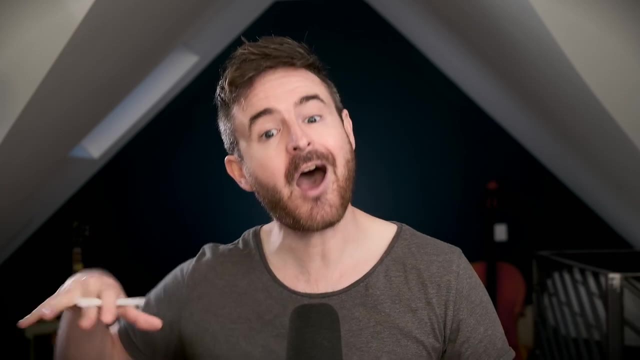 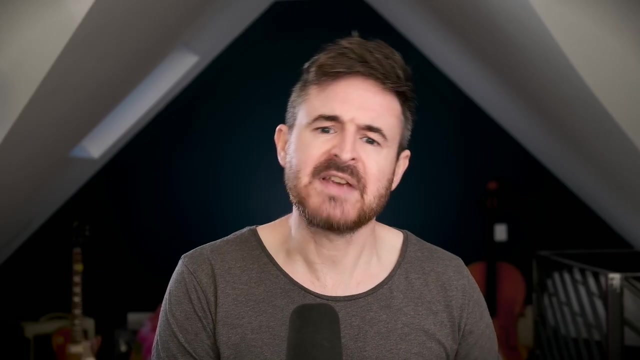 happy people, Anna Beck, would be all of the things in the whole domain that aren't in that set. So in that case, Kath, So the complement of the happy people would be the unhappy people. So this kind of corresponds to negation. Finally, the power set. This one's a little. 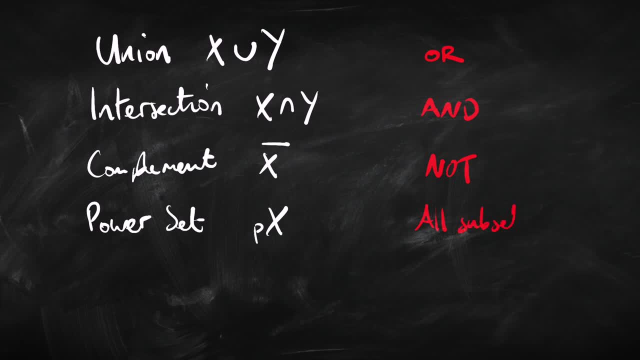 bit more complicated. Finally, the power set. This one's a little bit more complicated. The power set of a set is all of its subsets. Okay, that one's a little bit more complicated. so let's look through some examples. Okay, suppose we have these two sets. There's x. 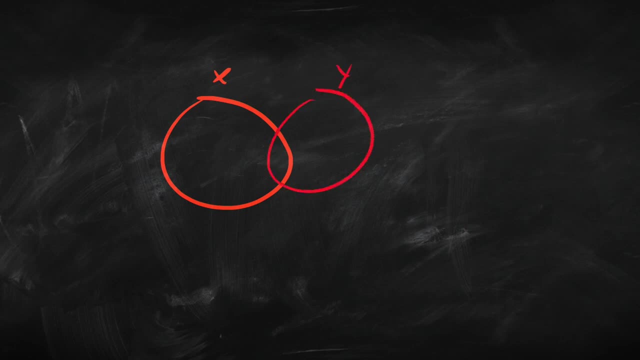 and there's y. Okay, I'm not drawing out all the things in them, I'm just kind of drawing them as circles. The union of those two sets is all of the things here plus all of the things here. The intersection of those two sets is everything in the middle here. 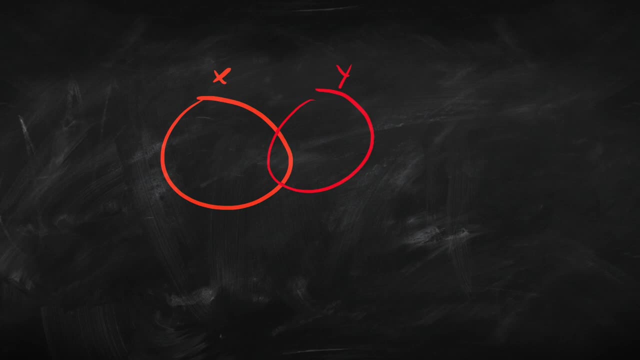 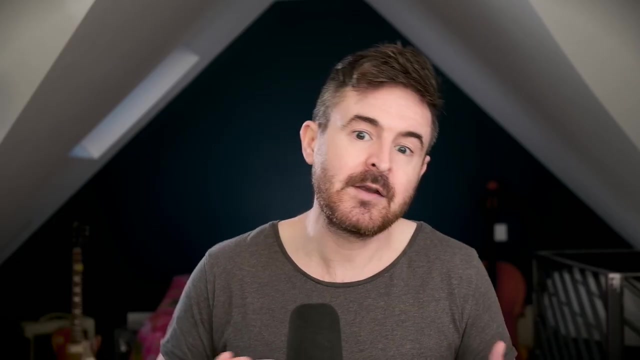 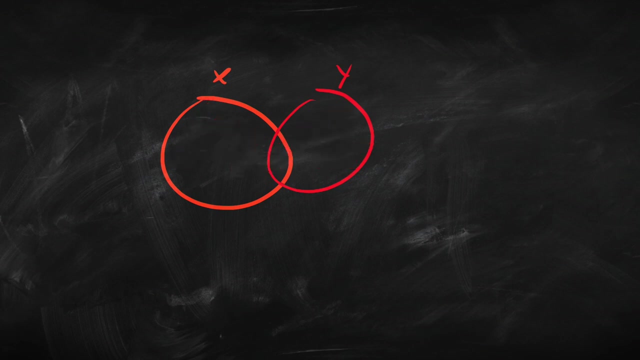 And the complement of those sets. well, the complement of x would be everything out here, everything that's not in x, And we can use these kind of concepts in conjunction. Okay, so the union of the two sets is this, So the complement of the union of the sets. 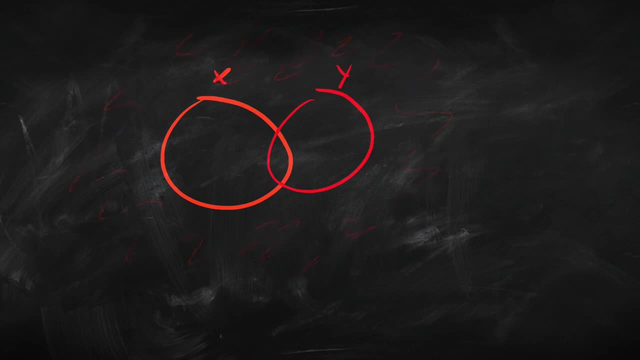 is everything that's not in either of them. The complement of the intersection of those sets is everything that isn't in both of them. So that is all of this over here, plus all of this over here, but not this bit in the middle here. And finally let's get on to the power set. 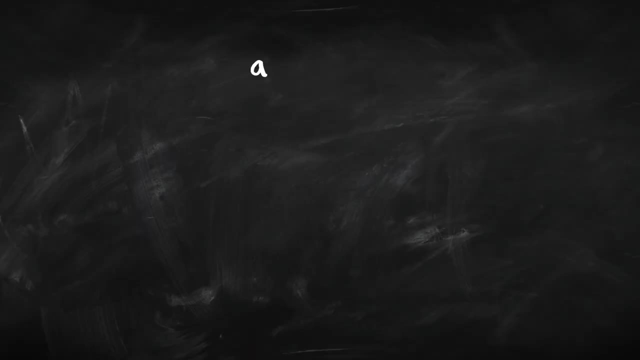 This is the one that's a little bit more tricky. So let's start off with this set from before, a and b, And we're going to try and look at all the sets that are subsets of this. So we're going to calculate the power set of a and b. 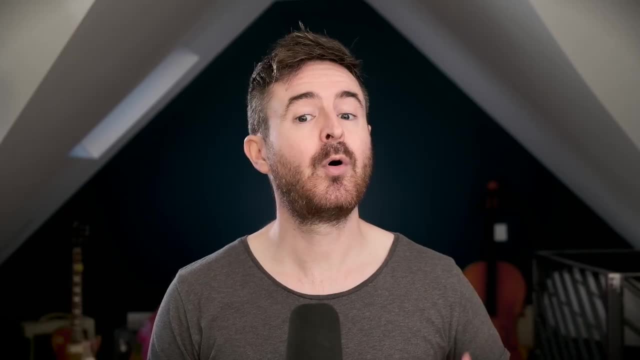 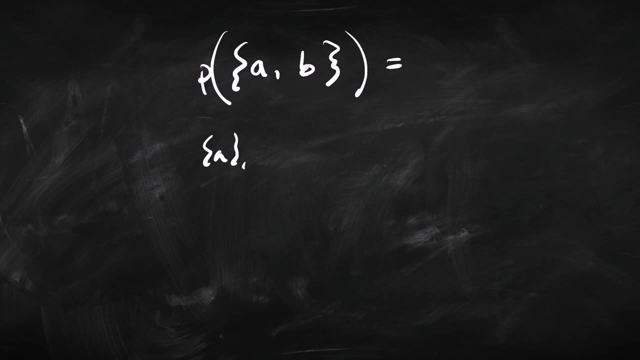 Okay, so we're going to list out all the sets that are included in this set. Okay, so you might go like this: Well, that's going to be a, b And remember, subset also includes the case where they're the same set, So we'd also better have a and b, Okay, and I put them in a. 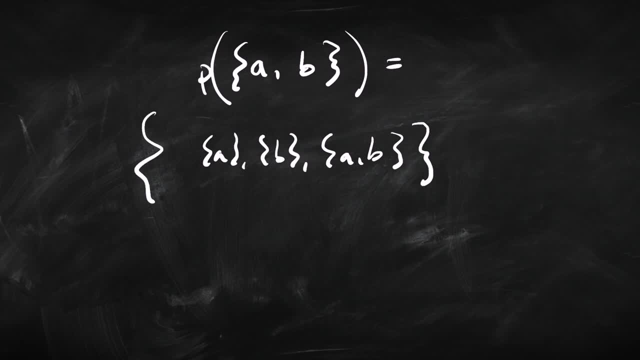 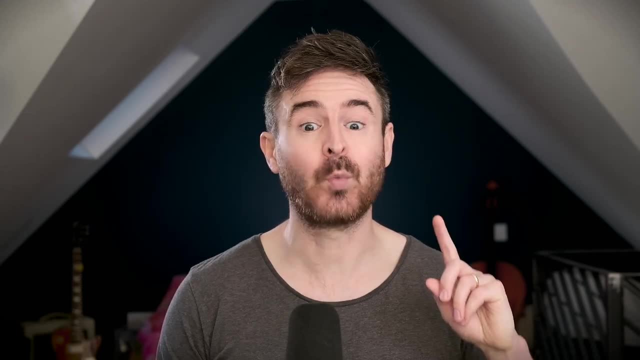 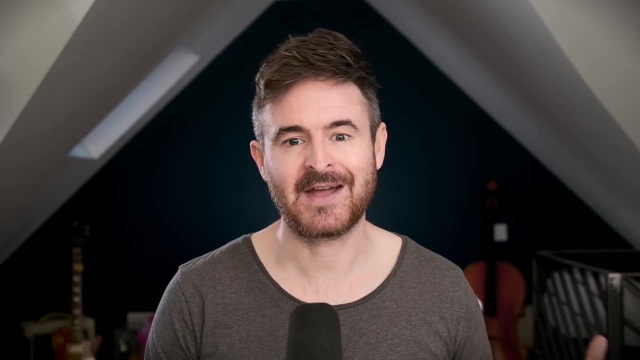 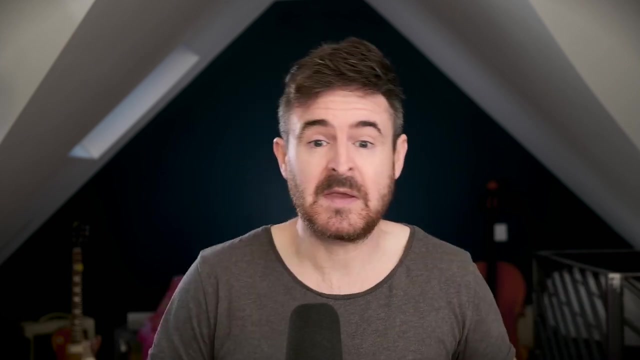 All subsets of it? Not quite. There's one I'm missing out, and that is the empty set. Okay, why the empty set? Well, think back to that definition of subset. X is a subset of y. if everything in x is also in y, Another way to put it will be: there's nothing. 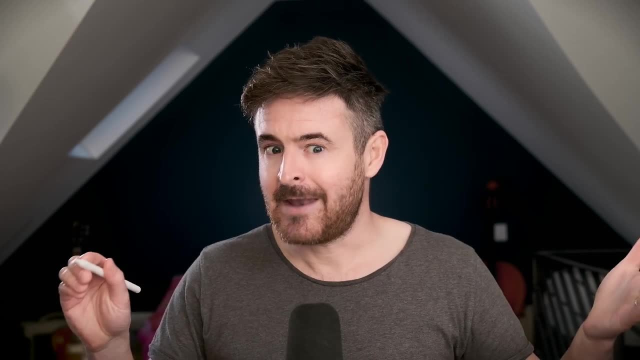 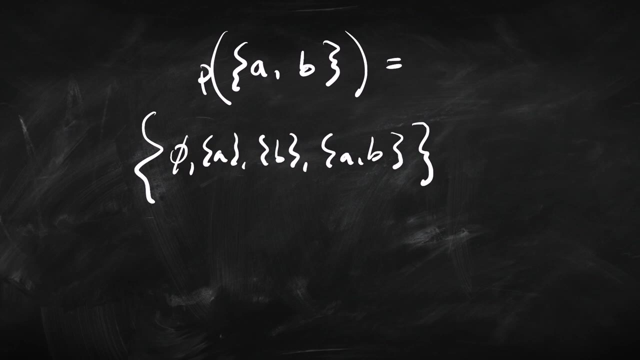 in x that isn't also in y. Now think about the empty set. Is there anything in the empty set here that isn't up here? Nope, because there's nothing in the empty set, So there's nothing here that isn't here. so the empty set will be a subset of this set. 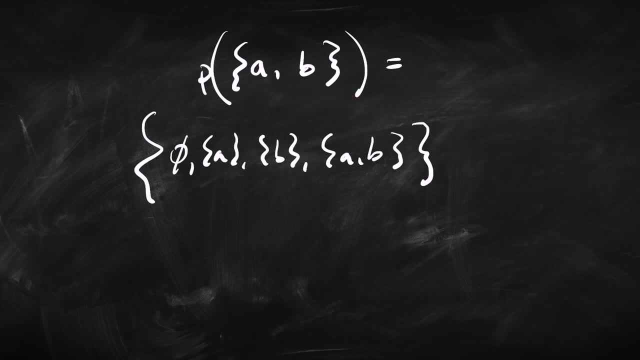 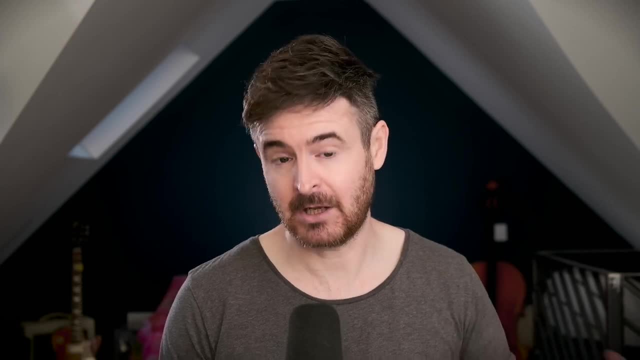 And, if you think about it, there's nothing special about that set that makes that the case. That's a completely general fact about the empty set. It's a subset of every single set, including itself. So whenever you're calculating the power set of a set, you always need to. 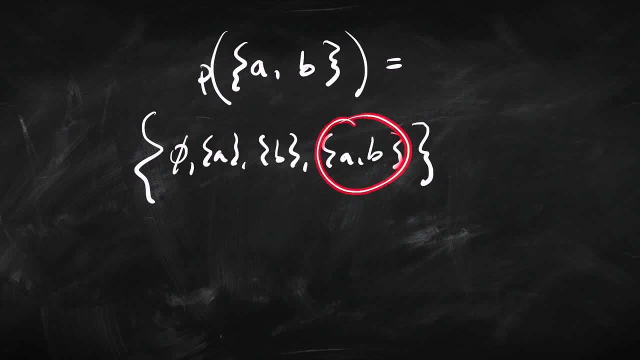 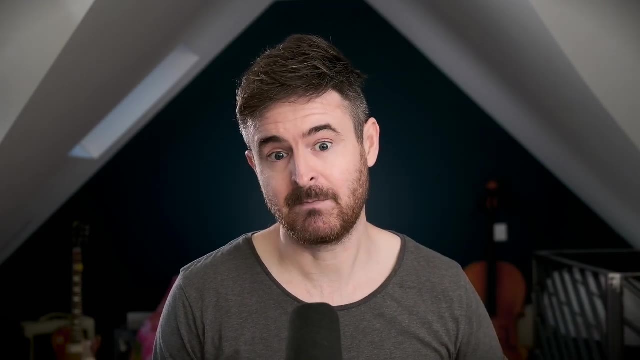 include the empty set. You always need to include the set you're starting off with with, and then all of the other proper subsets that go into the power set. Let's move on. There are different ways of writing down a set, So writing down the members of the set. One way is 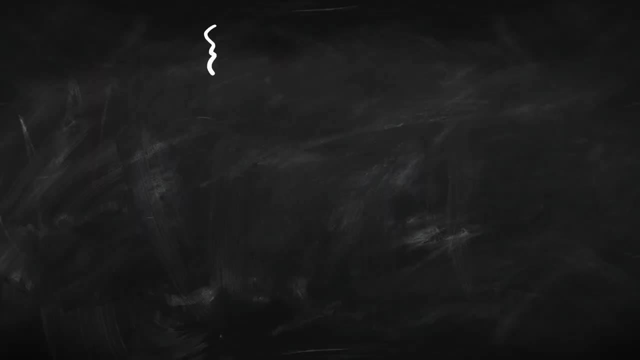 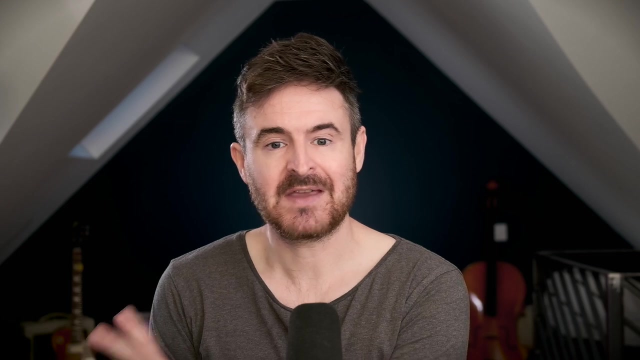 the way that we've been doing it so far, by enumeration, by listing them out, So we could say there's Anna, there's Beck and there's Kath. But sometimes we don't want to list out everything in the set. I mean, that's fine for just three things, But what if it was an infinite number? 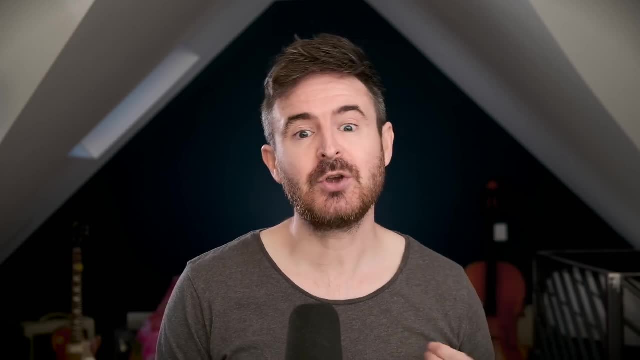 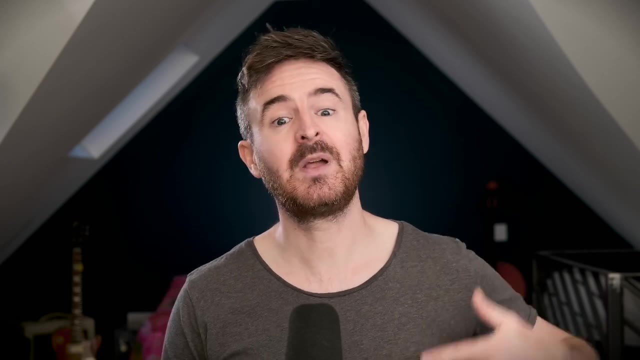 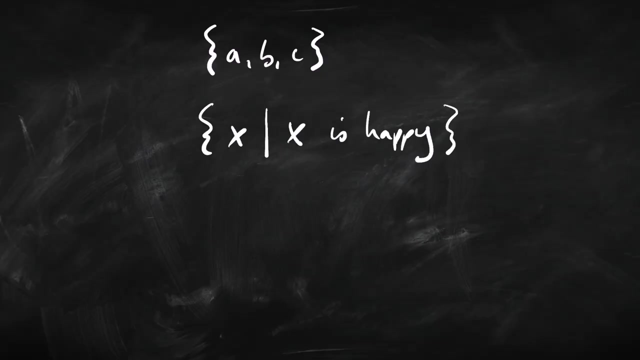 of things like the numbers or whatever. OK, so we can also use what's called set comprehension notation, And what we do there is we specify some condition or property for being in the set and we do it like this. OK, so what we've got there is: we're looking at the set of all things X, such that 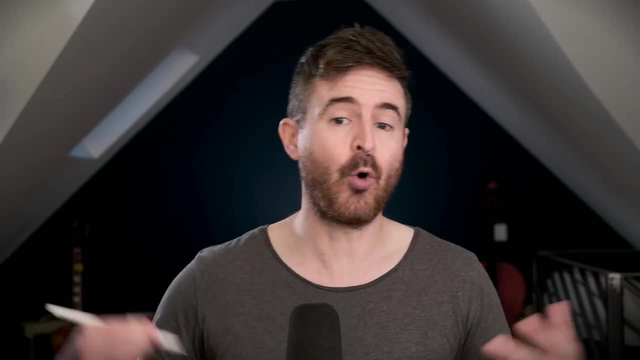 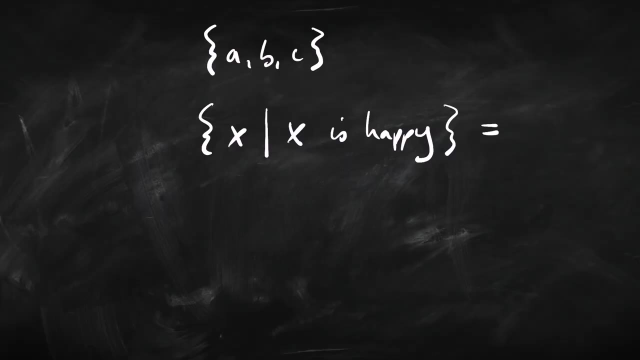 X meets this condition: being happy or being a person or being a natural number or whatever. OK, so in our previous example, this set would be identical to Anna and Beck, because they're the happy people. OK, this is a really useful way of specifying what gets to go into the set without writing them all out. 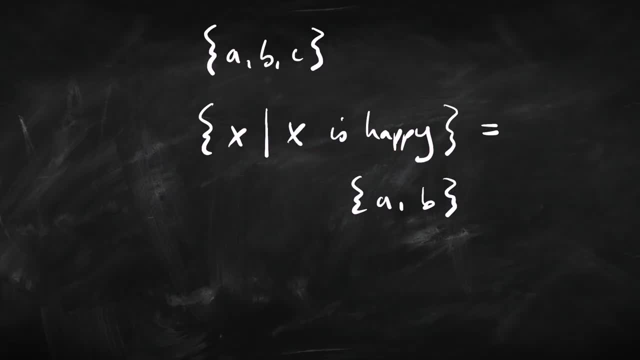 So we give some condition over here on the right. we write the full thing out by saying we're looking at the set of things X such that X is happy, or we could say the set of all pairs X and Y, such that X is taller than Y, Or whatever. OK, 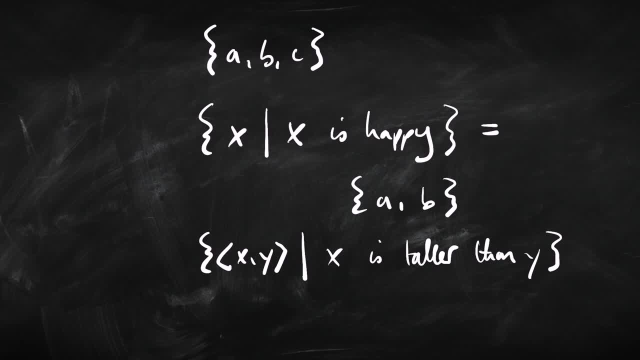 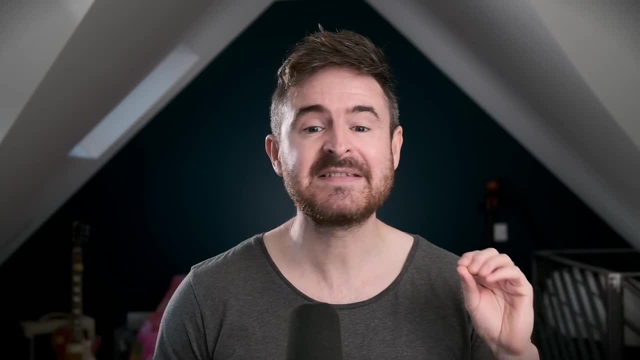 This gives us the full thing. We can use all things on the set, But we don't want to put the us a really useful way of specifying sets- sometimes really big sets- without having to write everything down, and you're going to see this notation come up quite a bit. okay, guys, that is it for this.